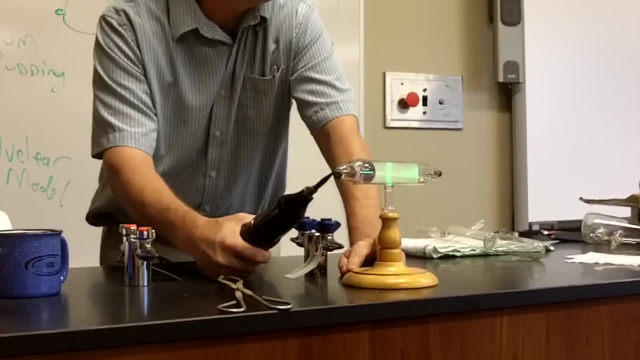 It's pretty cool. I actually can't see it from my side, but I assume you're seeing a straight green line mostly. Why can't you see it? Because I'm looking from behind. I'm a little bit confused. You're looking from behind. 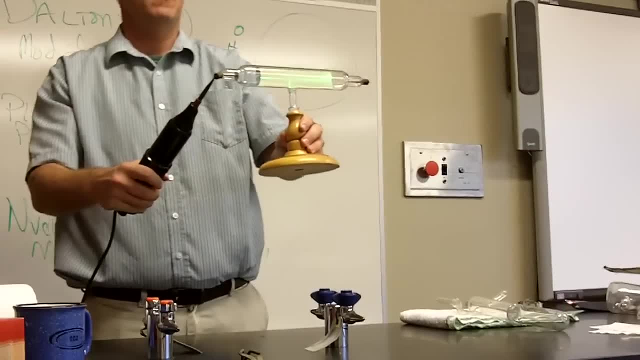 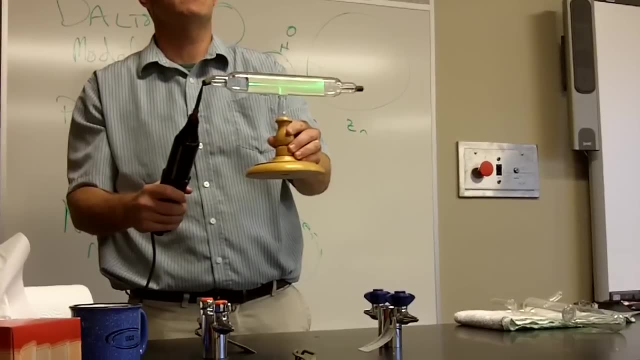 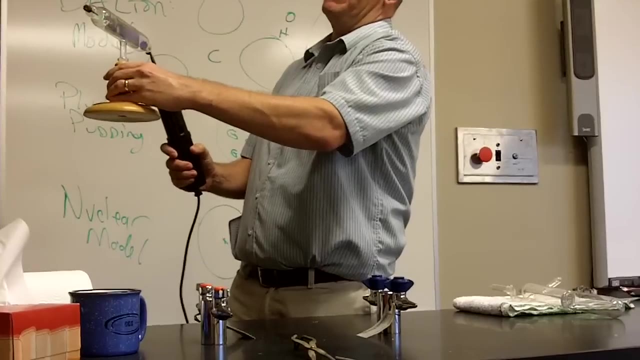 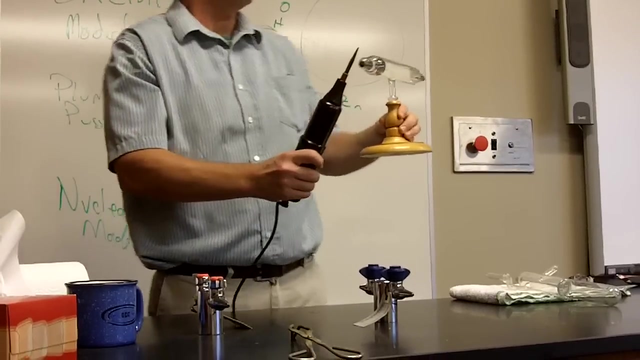 Yeah, I'm a little bit confused. cool, I actually can't see it from my side, but I assume you're seeing a straight green line, mostly because I'm looking from behind that. white screens only on the front. it's set up to be viewed from one side only. all right now. 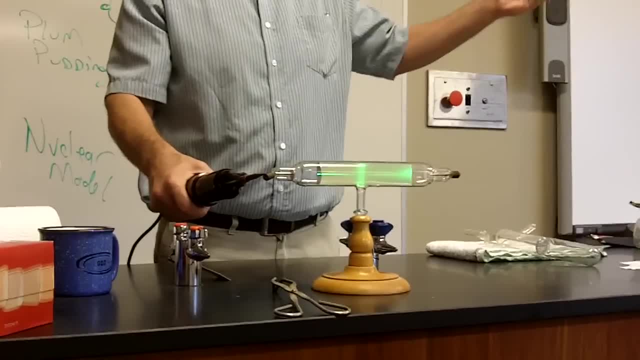 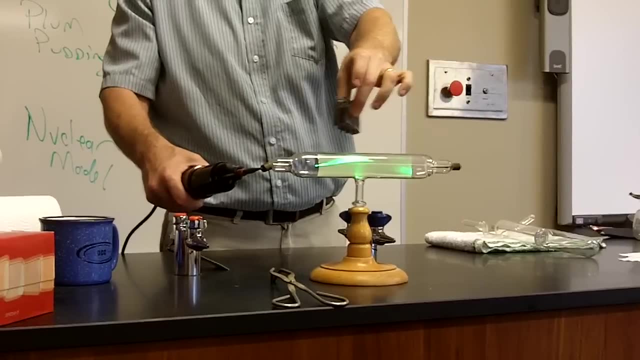 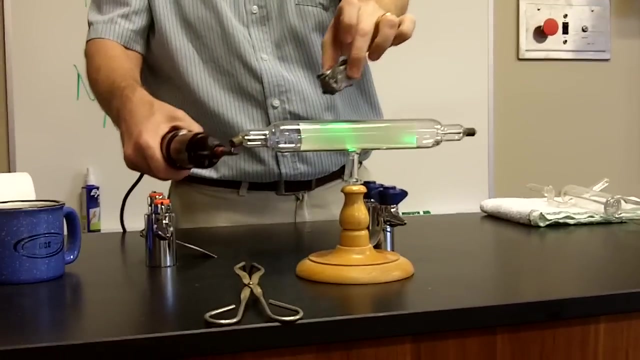 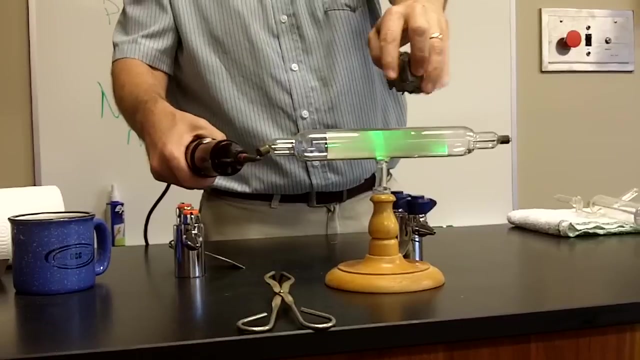 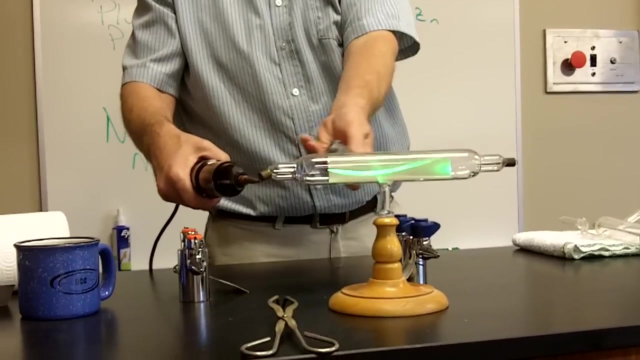 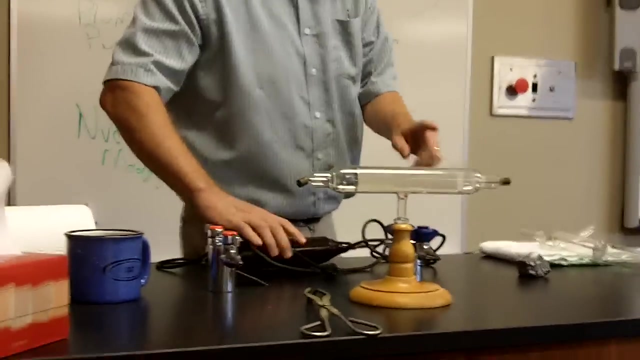 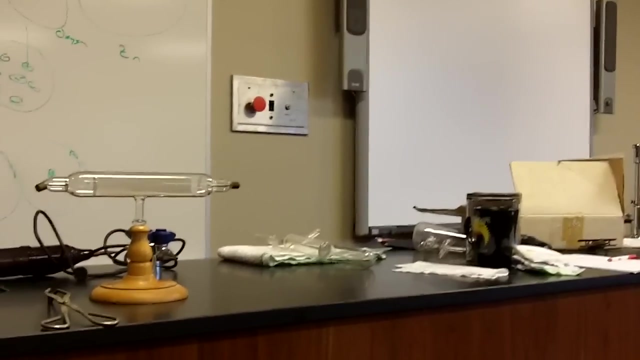 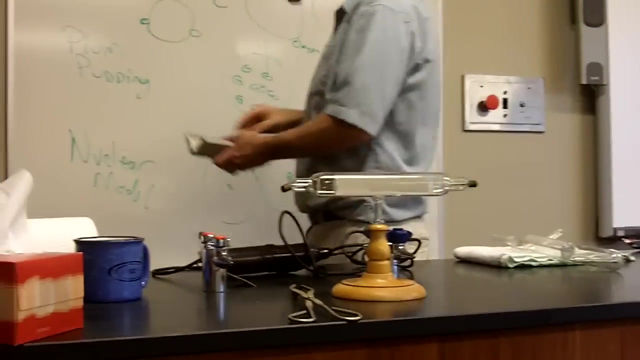 this is kind of interesting. watch this is anything happening. what's happening? hey, it's following the magnet, reacting to the magnet, deflecting the magnet. okay, so that's kind of interesting. keep that going. I got a one other thing to compare that to. I have light here and I have, I'm gonna 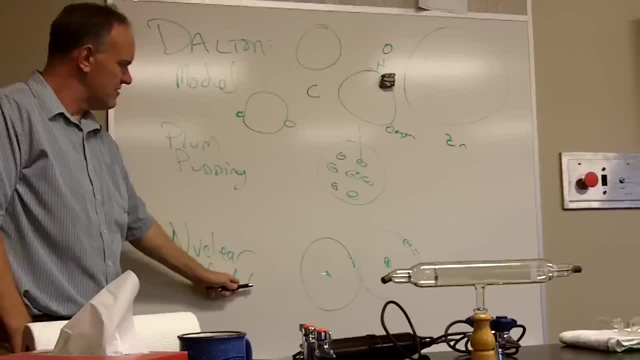 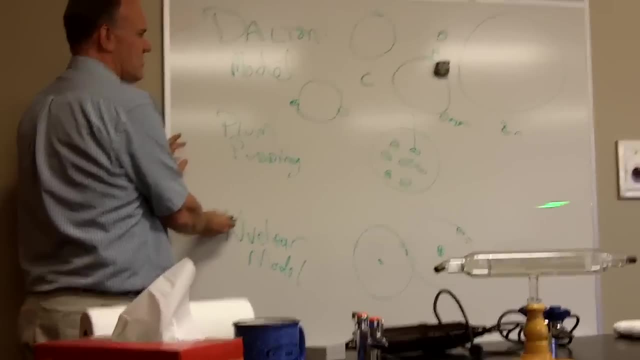 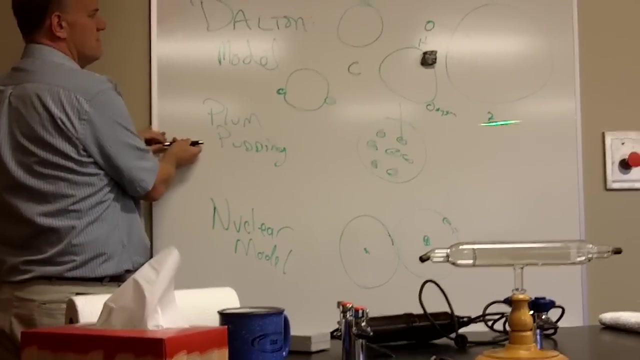 pass this light. it's a laser light, the green laser light on bit. that don't feel me. no, there we go see it. you see that uh got laser lights. is there? what'll happen to it? when I get it close to the magnet, deflect away, he says. 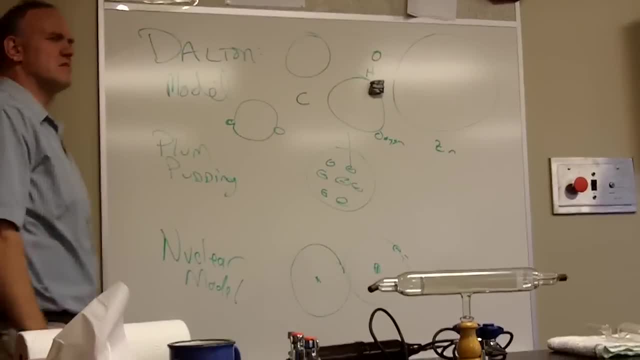 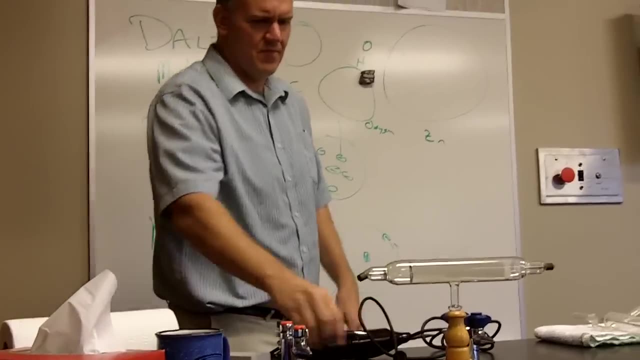 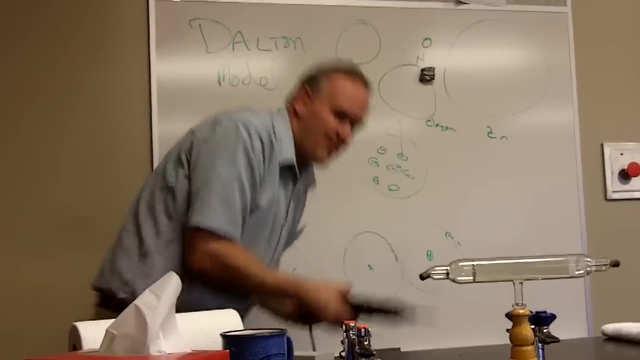 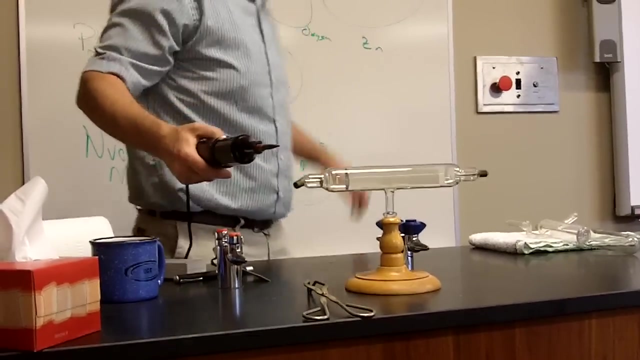 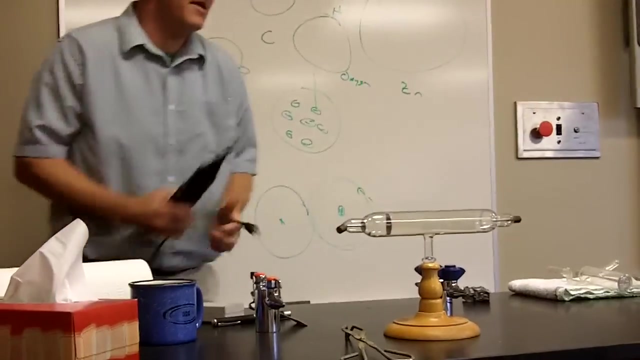